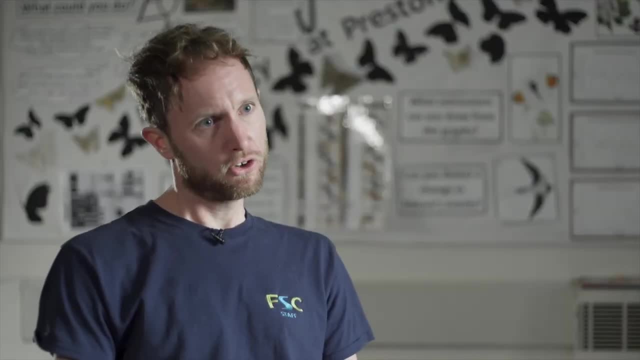 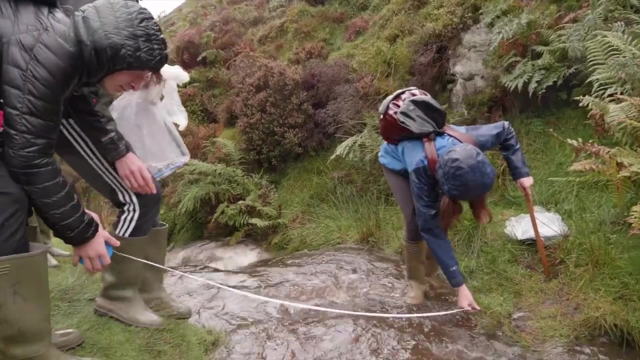 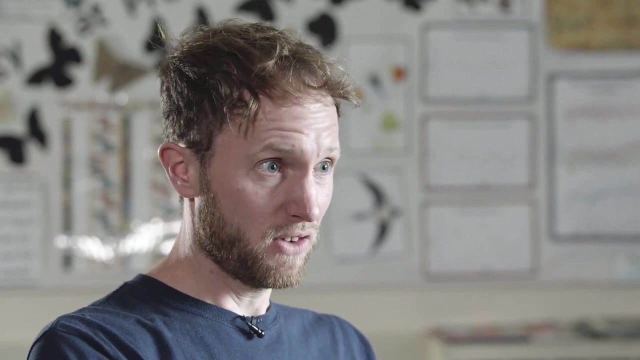 learn in lessons. It's really important to question students consistently and constantly to apply the methods that you use in the classroom out in the field. It's also important to try to use exam style questions out in the field to try to develop that connection between what they're doing in the field and how that 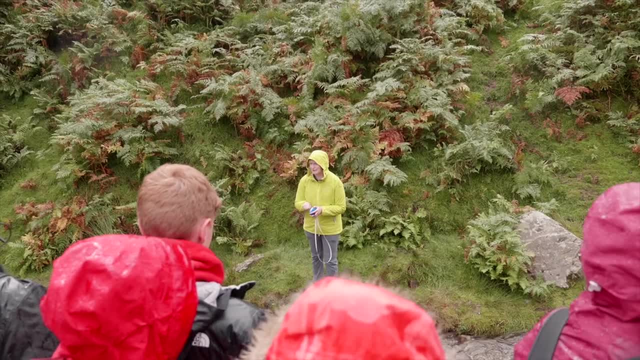 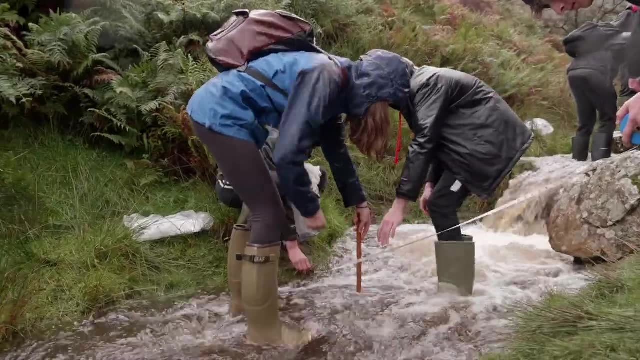 might be applied during the assessment. When we were at the river side, we'd measure the width of the river by using the tape measure, and then we'd measure the depth using a 30 centimeter ruler. and we'd measure the depth ten times to make sure we'd get a range of views. so we get. 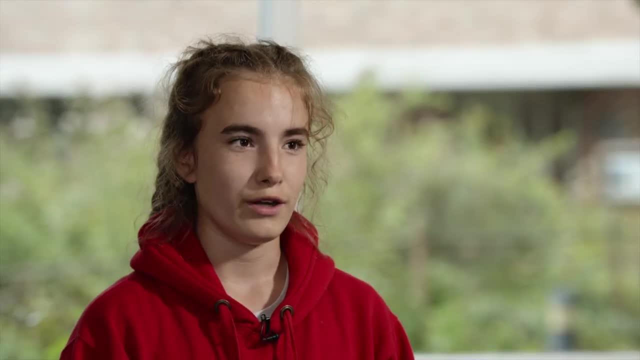 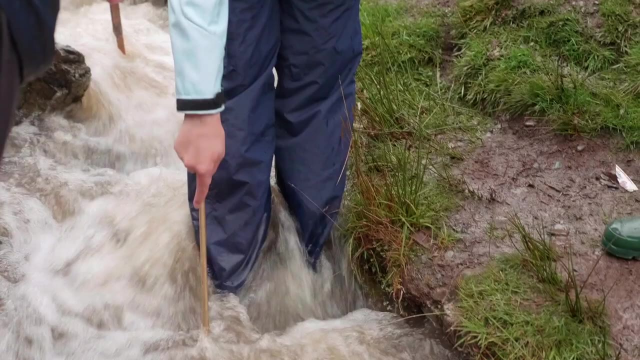 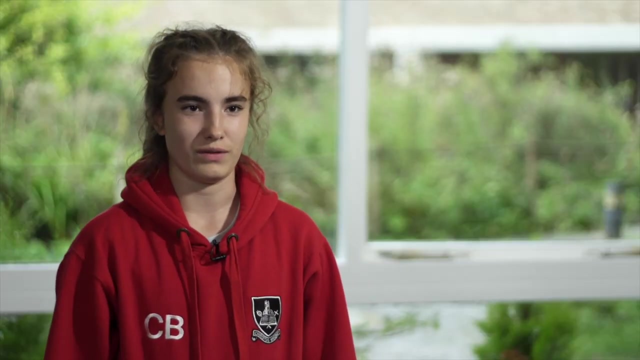 a nice average. and then to measure the velocity of the water, we used a hydro prop which we'd submerged in the water, which had an impeller attached to the bottom which would move across the bar, and we timed how long it took for the impeller to move. that would give us the velocity in which the river was moving. 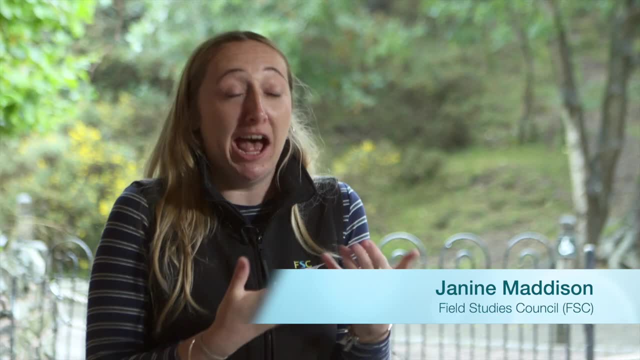 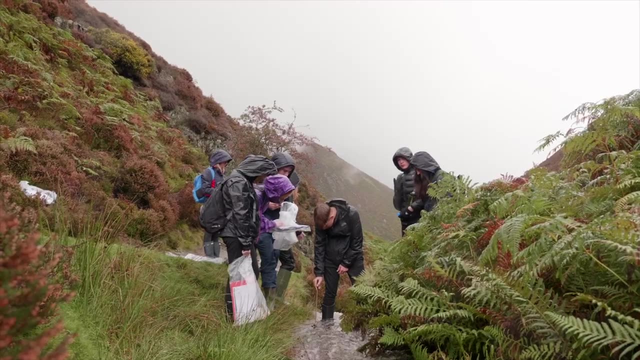 I think today the fieldwork that the students have done has been quite challenging for them due to the weather, but I think that that's important, because the data that they've got today might not be what they've expected and their results might be a little bit different, and it's really useful for 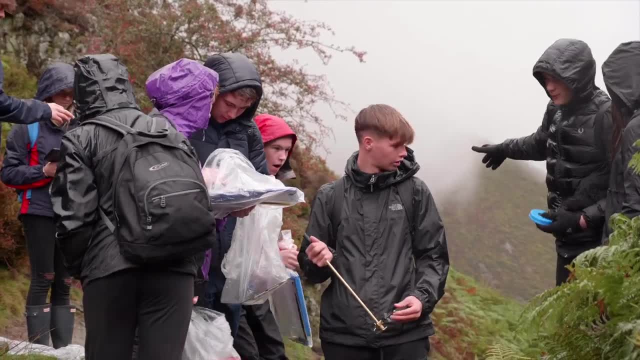 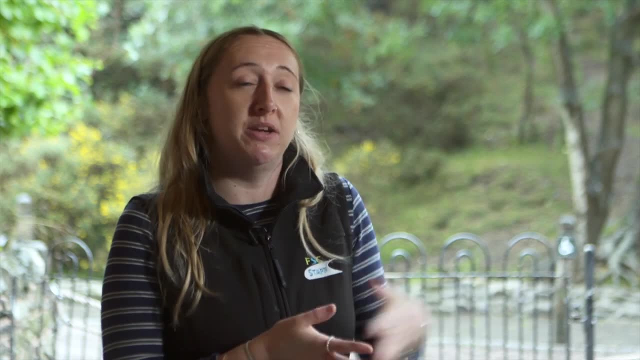 students to be able to think about why that data might be that way. so today they might be talking about reasons why their rivers data might be not what they expect, and that's gonna be important when it comes to their unfamiliar fields work when they're provided those contexts in the exam to really think. 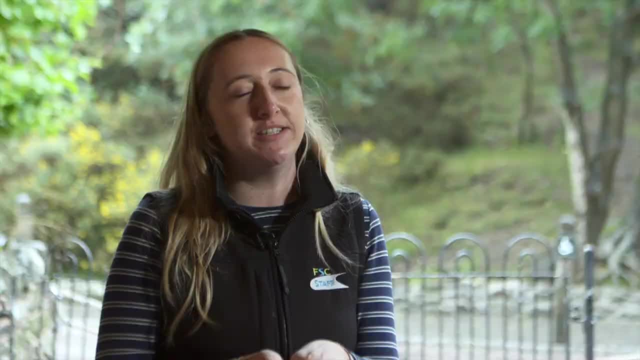 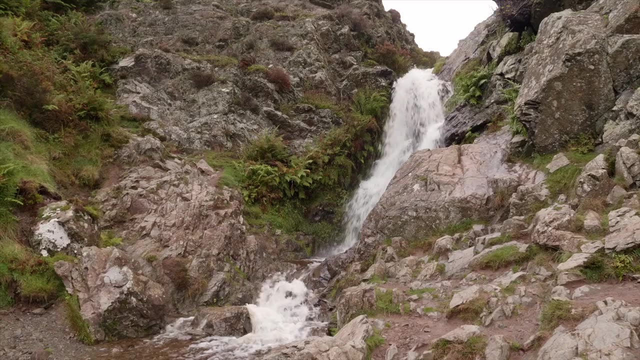 about the data that's in front of them, the context that it sits behind. The most memorable thing about today was probably seeing the different features in the river. so there's the waterfall, which was pretty big at the top and that that was pretty good to see, I think, seeing, like, the force of the water as you went down the 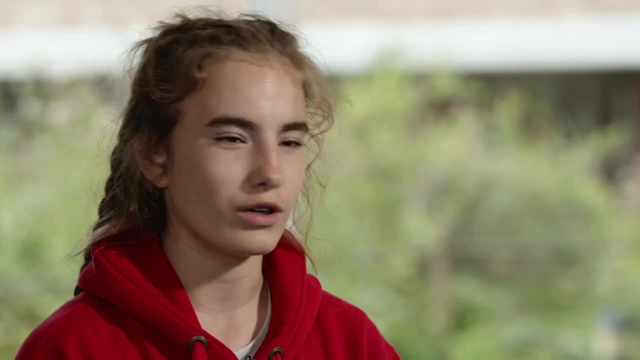 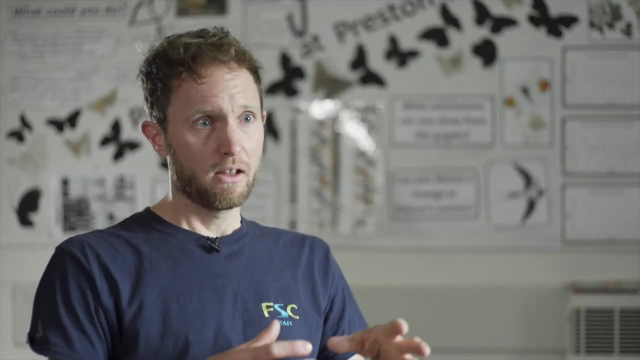 river, like seeing how much it started to build up and it was quite strong, like when you had to walk through the river. you could feel it really pushing you along the stream. It's important to create memorable moments throughout the fieldwork day and give students that sense of awe and wonder, and Carding Mill is a great location to 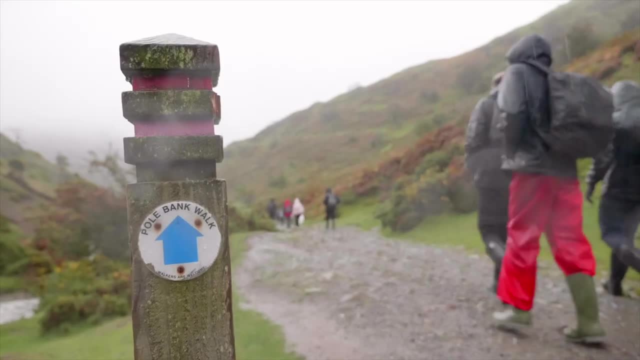 do that. It's inspiring young geographers out in the field.